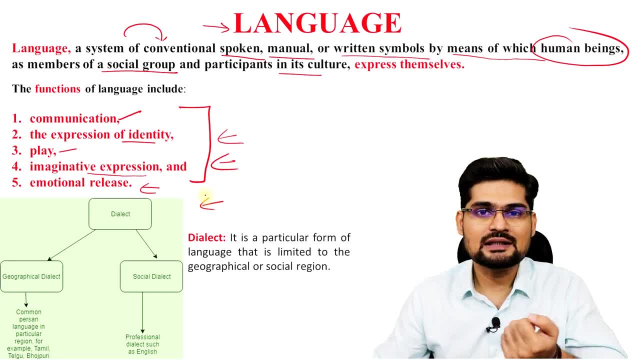 there is a spatial pattern of languages in the world. it means language changes from location to location. and when we say there is a locational aspect, a spatial aspect in the language, it becomes purely human geography concept. right. so understanding this particular flow diagram, there is also something called dialect. and what is this dialect? one is called geographical dialect. 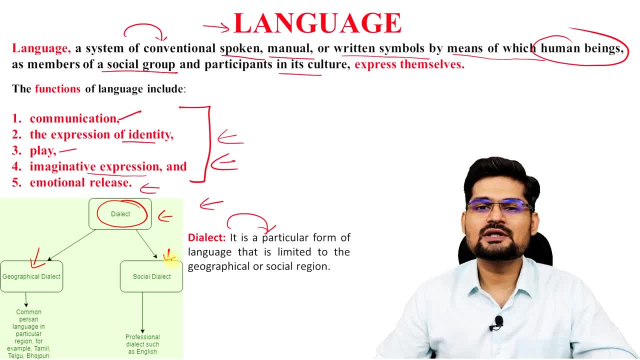 and one is called social dialect. so dialect is basically a particular form of language that is limited to a particular location or a social region. right, and when we say social region, it means a region dominated by a particular group or social group. right, that's where a dialect 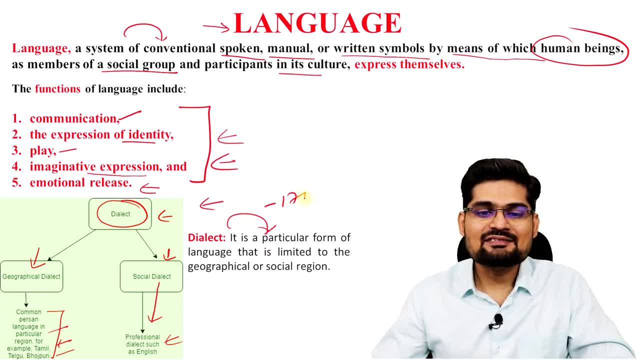 forms. and also what we know is that more than 1700 dialects exist in india. right, so we can say that there are several dialects. that is basically talking about a division in the space, right, in terms of linguistic plurality, language is a plural concept, right, so there is a plurality in the language across the space, and that's why we say: 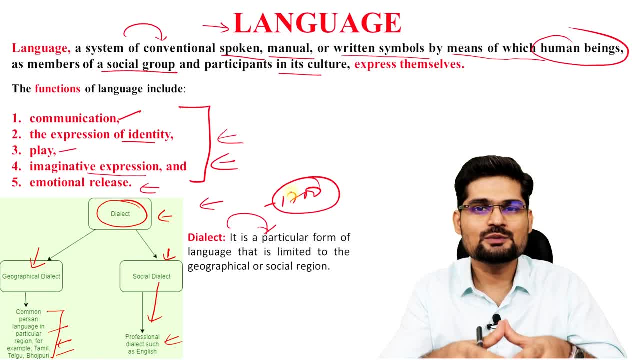 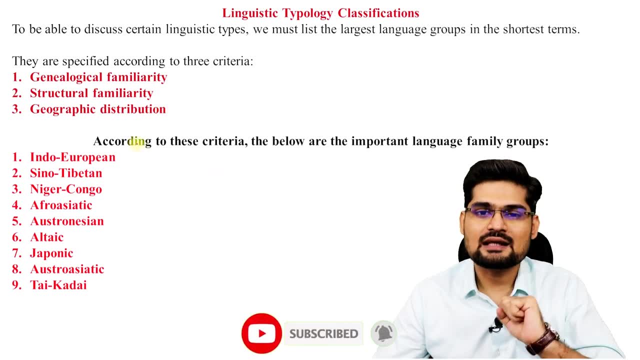 that language is also related to perspectives in human geography. so now let's elaborate and understand this linguistic typology classification. how have these languages been classified? in a spatial connotation, so what we observe here. to be able to discuss certain linguistic types, it's very important to understand the list of these large language groups. so they are specified according to. 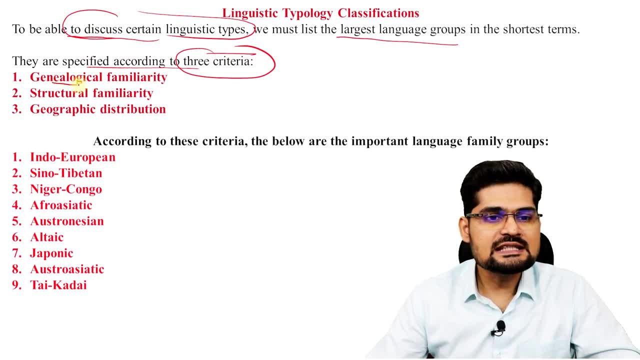 criteria. and what are the three criteria? one is called genealogical familiarity, then structural familiarity and then geographic distribution. three things are very important. one is on the basis of genealogy, the genesis, the origin. the other is on the basis of structure, the composition and structure of a language, how it is built, what is its grammatical structure right. and the third is: 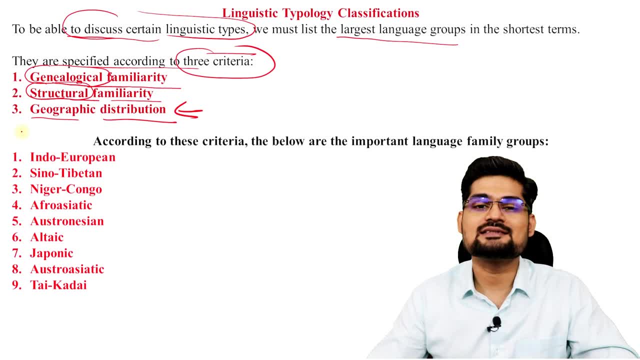 geographic distribution of that language, and that is where we are concerned, right? so, according to these three criteria, the below are important language family groups across the world. right? so what you observe? indo-european language, sino-tibetan language, niger-congo language, afro-asiatic language, austronesian language, altaic language, japanic language. 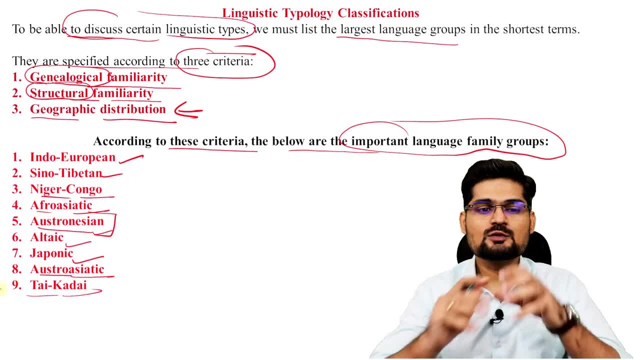 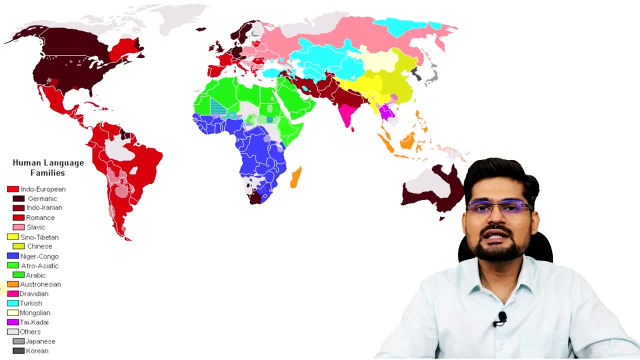 austroasiatic language and then thai kadai, so we have almost nine major linguistic groups across the globe, if you observe as a spatial pattern. so what you need, we need a world map to locate them. in this world map there is a very interesting colorful spatial pattern emerging out of languages. 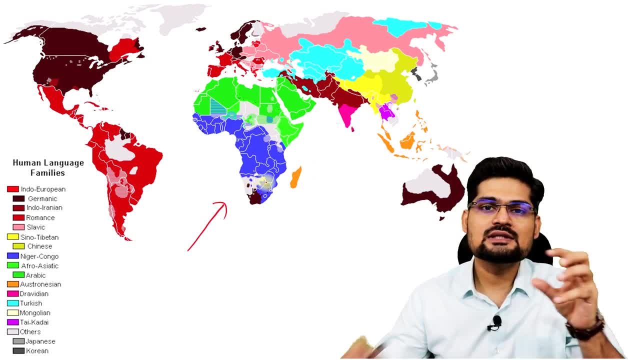 and that's why we say that geography is about the combination of these several attributes. when we say physical part, then it is physical geography. when we say human attributes- for example, language we are studying right now, that's a human attribute- also makes a spatial pattern in human geography and that is how it's visible on the map. 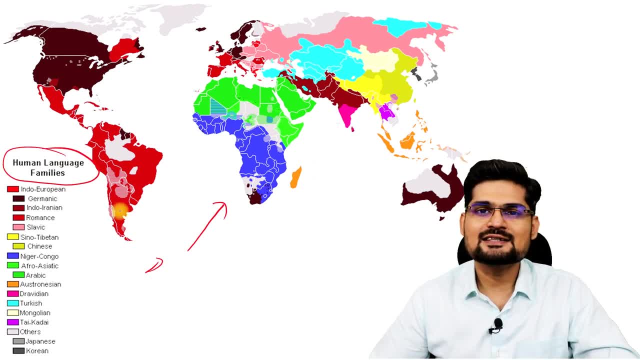 so, if you observe this map, you have human language families across the continents. so you observe indo-european, in which you have germanic, indo-iranian, romance salvic, then you have sino-tibetan, in which you have chinese, then you have niger-congo. this blue color in covering the 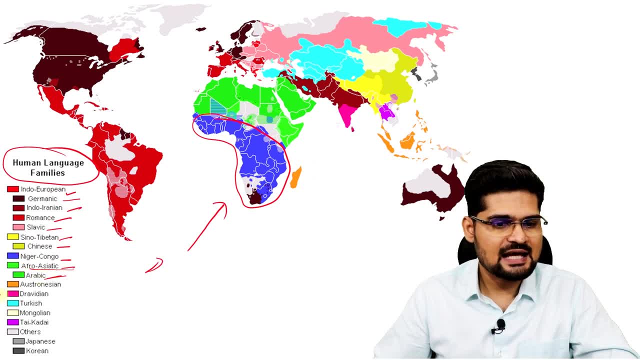 entire africa and apart from that, we have afro-asiatic as well as arabic language as well, under afro-asiatic, if you see, then austronesian, then you have dravidian, turkish, mongolian, tai, kadai and others, for example, japanese and korean right. so you observe this, various types of languages groups across the world, which are two languages based on their следующing cultures. about the African islands, you observe indiabetic, indiabetic and Sino-bibliotic and Indo-european. then you have China and Chinese. then you have checked out the Indian and African and the African. 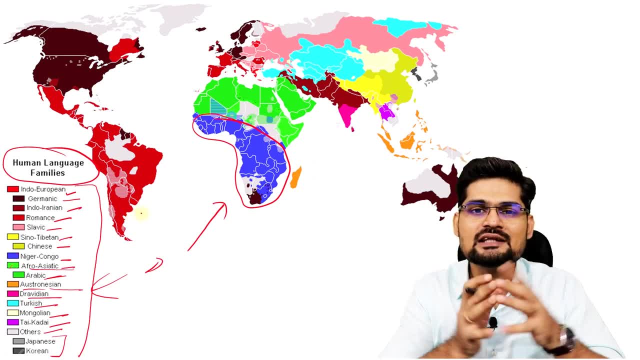 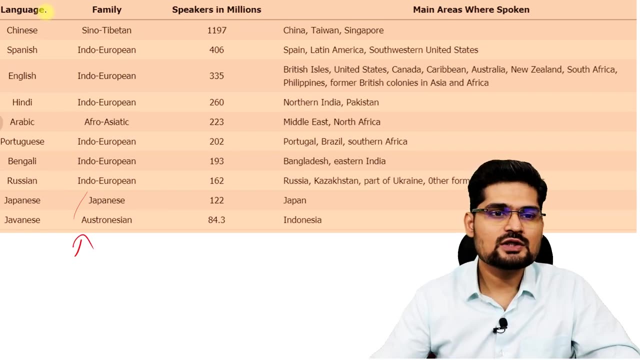 creates an interesting colorful pattern if we really want to draw a map of different languages. it's looking so colorful. it means the world is diverse in terms of language, in terms of spatial pattern, and that's why it's also important to understand the spatial pattern through the data. so what? the 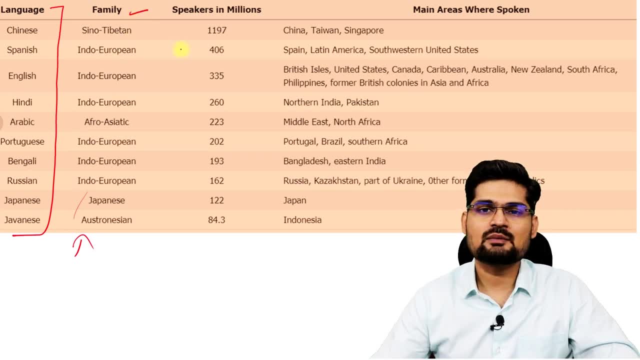 data we have. these are the languages, this is their family and this is the rough amount of speakers in the world in terms of millions. and these are the areas where we see is location or where we see is geography right. so, for example, Chinese is a sign of Tibetan language, which we say Mandarin, and then one one 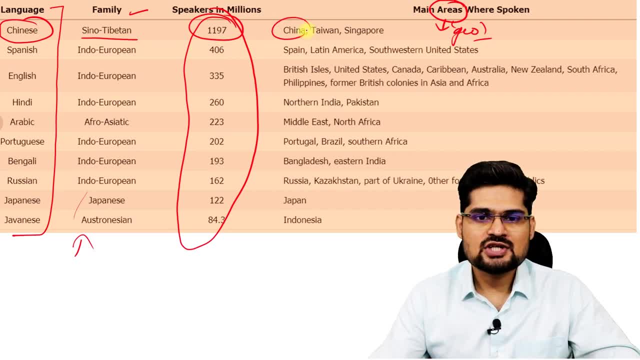 nine seven million people are the speakers of this, and China, Taiwan and Singapore is where Chinese is mainly spoken, right then Spanish, indo-european four zero six and Spain, Latin America, southwestern United States, English three, three, five, British Isles, UK, US, Canada, Caribbean, Australia, New Zealand, South Africa, Philippines, former. 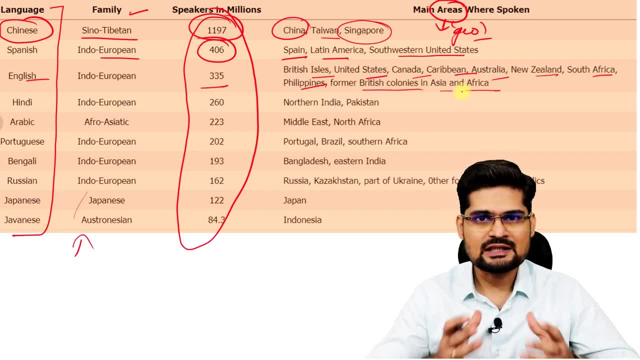 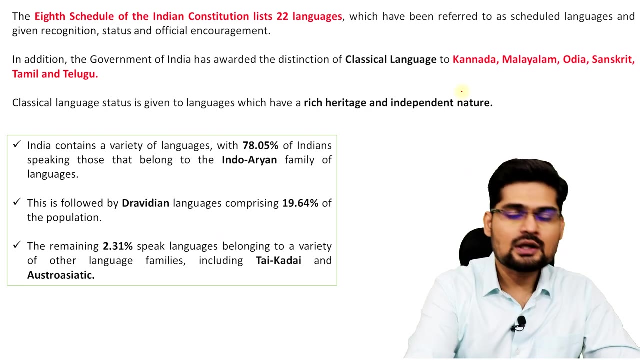 British colonies like Asia, Africa, in India, we, we also use English as one of the official languages, apart from Hindi, right? so what do you observe? these are spatial patterns of languages across the continents, right, and that's why we say it's purely a human geography concept. and now coming to Indian context, in our 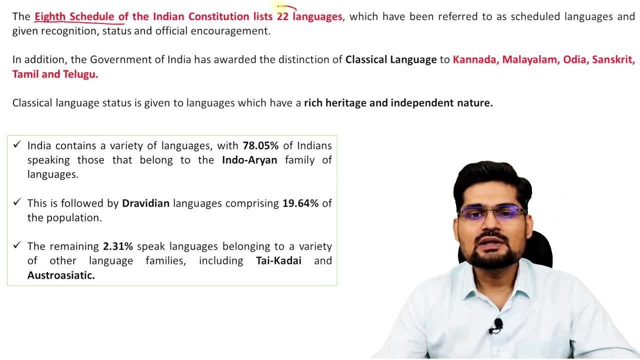 Constitution, in the eighth schedule, what we observe? twenty two languages are the premier languages or the prime languages in India, which is mentioned, which have been referred to as the scheduled languages giving recognition, status and official encouragement. right, but it's not just 22 languages, remember, there are more than 1700 dialects as well. right, and apart from this, our 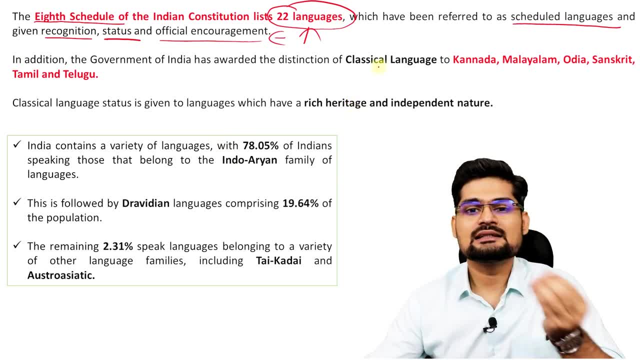 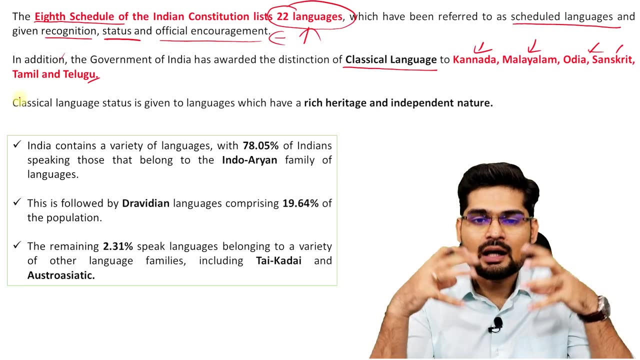 constitution also gives special, distinct class, that is classical language, we say, as to Kannada, Malayalam, Udaya Sanskrit, Tamil and Telugu, these are classified as classical languages in India, right so government of India has awarded this distinction. to actually understand their rich 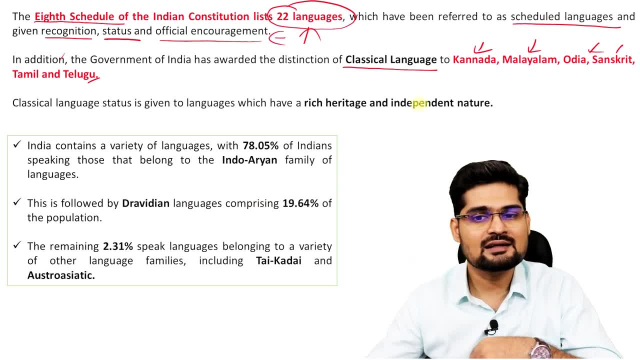 heritage. so this is part of rich cultural heritage in India and independent culture they have. these languages also relate to the independent cultural attributes as well, right, so, if you observe these facts here. India contains a variety of languages, almost 78.05 percent of Indians speaking those that belong to Indo-Aryan family language. then Dravidian languages are spoken by. 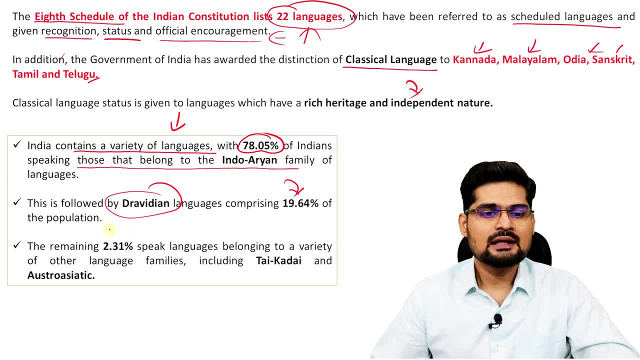 about 19.64, close to 20 percent of people, and then remaining is 2.31 percent, which is belonging to a variety of language families, for example, Thai, Kadai and Austro-Asiatic groups. right, so this is the linguistic diversity, or we say linguistic plurality, in India. in terms of data, you can. 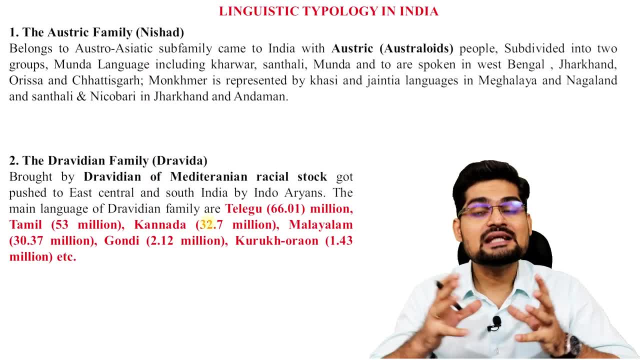 observe, right? so if you look here, linguistic typology in India, as we looked into the world pattern, this is what we see in India, right? so if you look here, linguistic typology in India, as we observe, the Austric family, which is also called Nishad family, belongs to Austro-Asiatic sub-family. 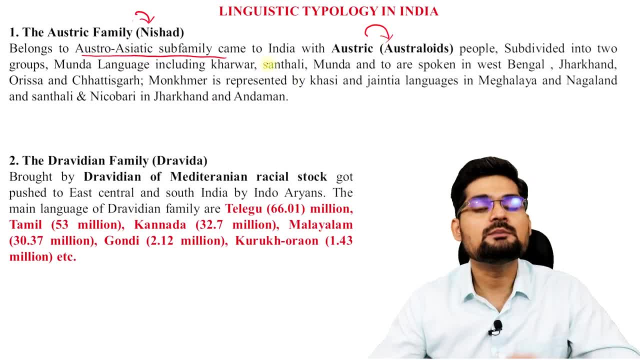 and it came to India with Austric or Austroloid people, if you have read about the race Austroloid race people. so it is subdivided further into groups called Munda language, into Kharwar, Santhali, Munda, and they have spoken where, in which parts of India- in West Bengal, Jharkhand, 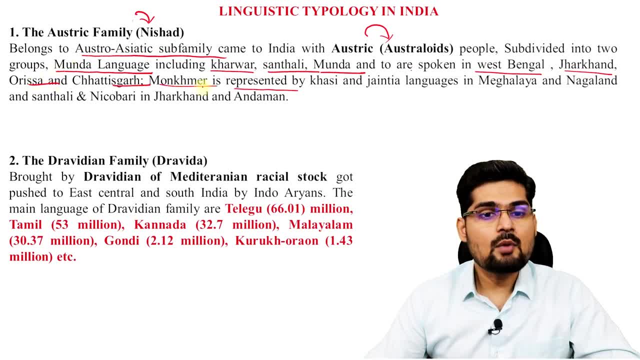 Odisha, Chhattisgarh. that is where it is spoken. then Monkhumar is represented by Khasi Jayantiya languages, where they are present in Meghalaya and Nagaland, and Santhali and Nico Barri we can find where in Jharkhand and Andaman. so they are all Austric family languages, that is. 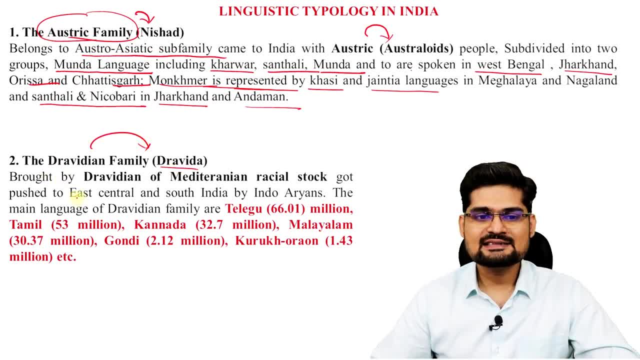 one type. then you observe Dravidian family, the Dravida that we say so, Dravidian of Mediterranean racial stock got pushed to East, Central and South Indian by Indo-Aryans. that is a proper popular theory which has also been criticized by many that this was a Max Muller's theory. but now the 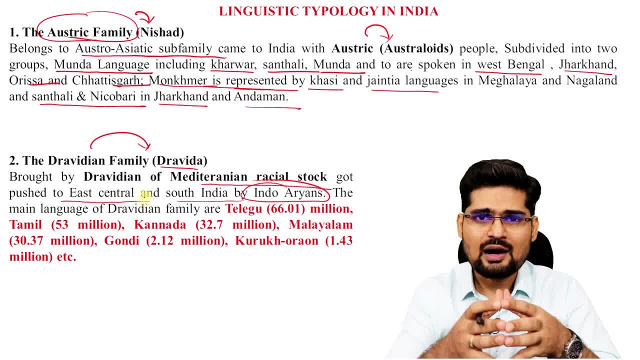 this theory is also under criticism, but for now, what we study is still. this theory holds true in many parts and is applied to the knowledge forms where we are studying. so we say that this is the truth, as validated by most of these scholars in that way. right so the main language of Dravidian 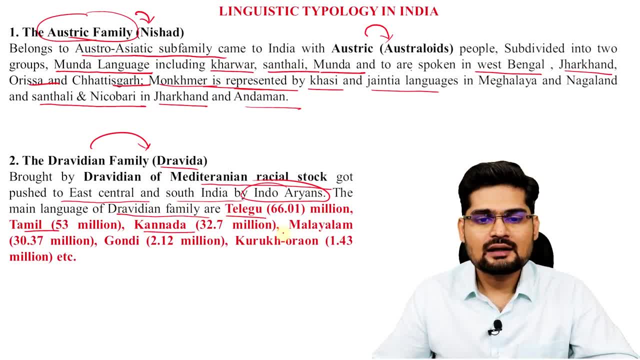 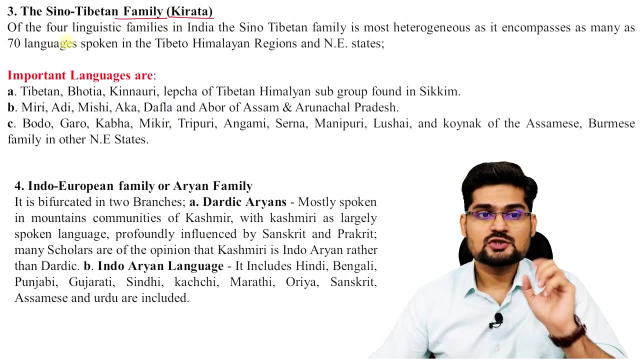 family are Telugu, then we have Tamil, then Kannada, Malayalam, Gandhi, Kuru, Kurao and several others. so these are all Dravidian family, Dravid family languages. then, if you observe, the other languages in India, the Sino-Tibetan family or, we say, Kirata languages. so out of the four linguistic families, 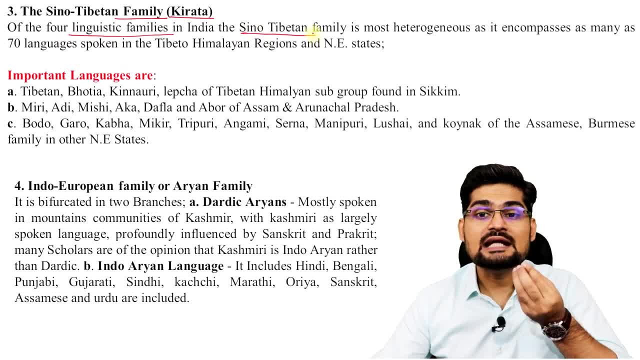 in India, the Sino-Tibetan group family is most heterogeneous group. why it is heterogeneous? it comprises of 70 languages inside this one Sino-Tibetan family. that's why it's called a heterogeneous group: combination of several small, small, small, small languages inside a huge family. 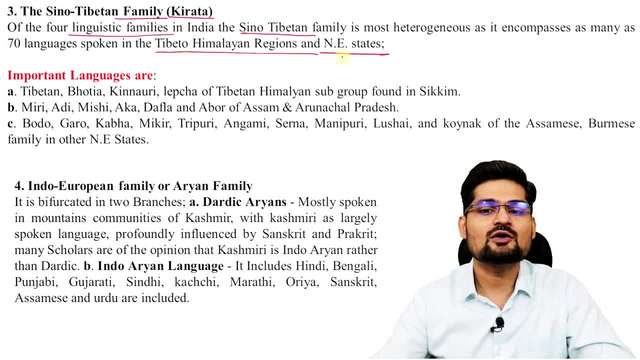 that is called a heterogeneous family. and that is called a heterogeneous family that is spoken basically in tibeto-himalayan regions and northeastern states in India, right. so important languages in Sino-Tibetan family, if you observe the list here: Tibetan Bhotya. 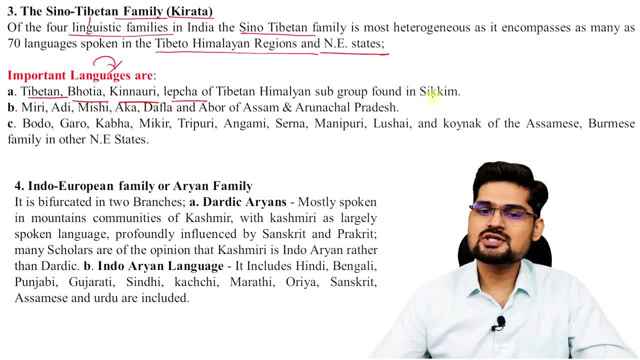 Kinnori, Lepsa, right, that is spoken in Himachal, in Ladakh and Sikkim. then we have Miri Adi, Mishi Akka, Dhafla and Abhor of Assam and Arunachal Pradesh. then we have Bodo Garo, Kaba Mikhir. 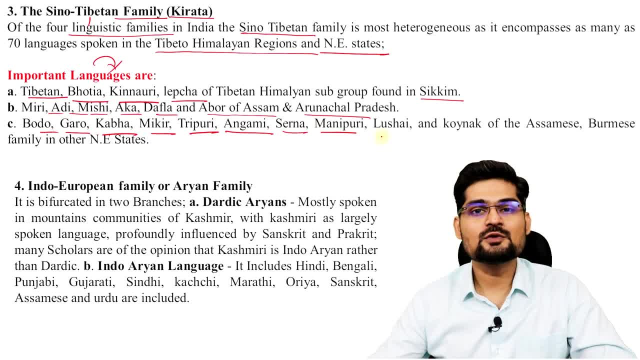 Tripuri. then we have Angami, Sarna, Manipuri, Lushai, Koinak of Assamese Burmese family that is in northeastern states in India, right, and then fourth family, the major family that we observe as a special pattern of languages in India, is Indo-European family, which we observe. 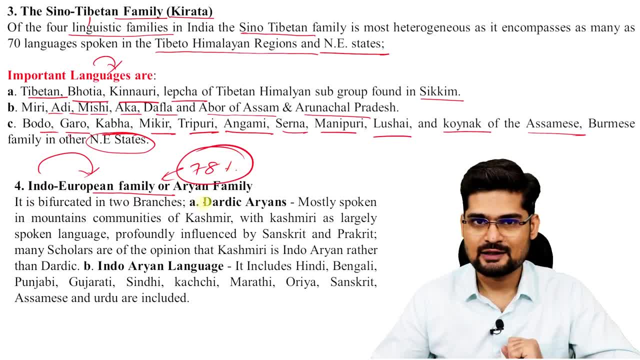 as 78% of India speaks this family languages right, so it's bifurcated into two branch. one is called Dardik Aryans. now, remember, Dardik Aryans, or Dardik Aryans, are those people who are mountain community, right, so they belong to Kashmir, specially in Kashmir areas, and 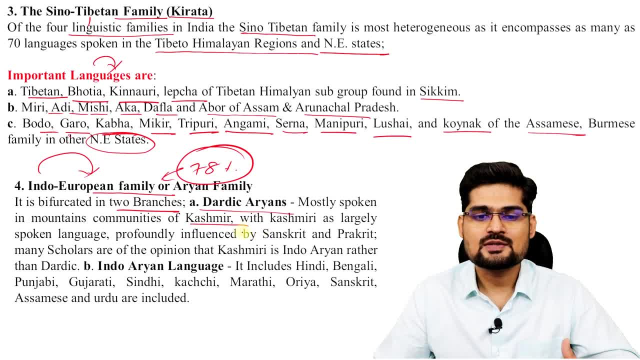 upper Himachal areas where you have Kashmiri as a major language. but remember they are profoundly influenced by Sanskrit and Prakrit, right, that's important to understand. and also many scholars are of the opinion that Kashmiri is also an Indo-Aryan rather than Dardik. but 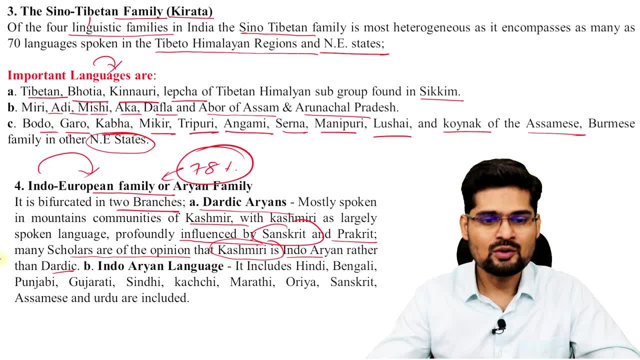 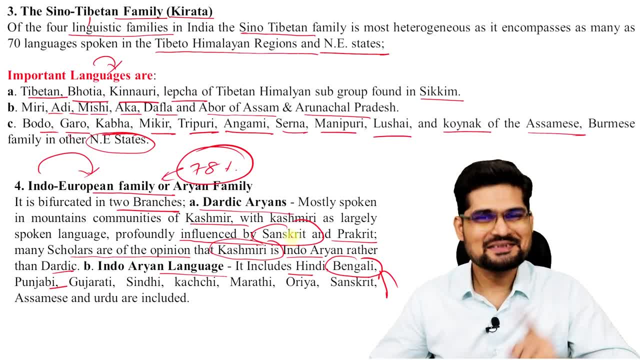 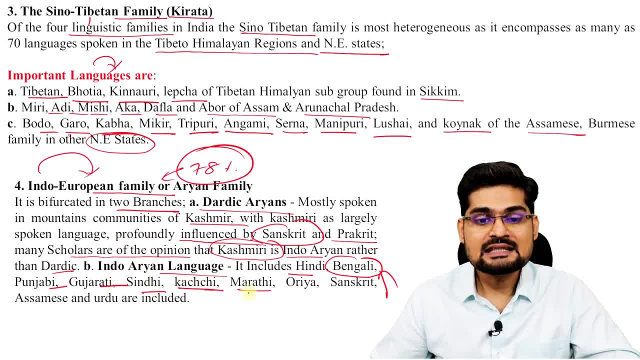 and also Gujarati, S, tranthiragi, Kanchi, Moongdada, Odaya, Sanskrit, Asamese & Urdu, which are included in Indo-aryan languages, right? so if you observe the list, what we say, that's a huge diversity. 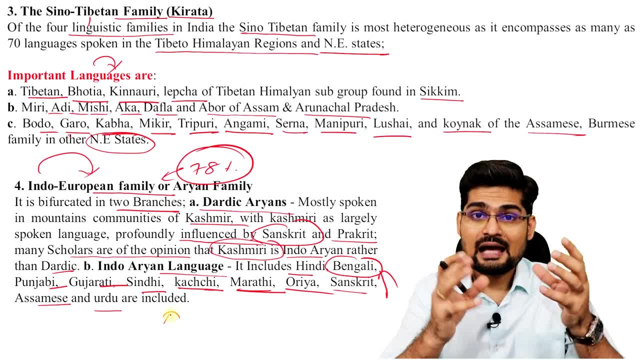 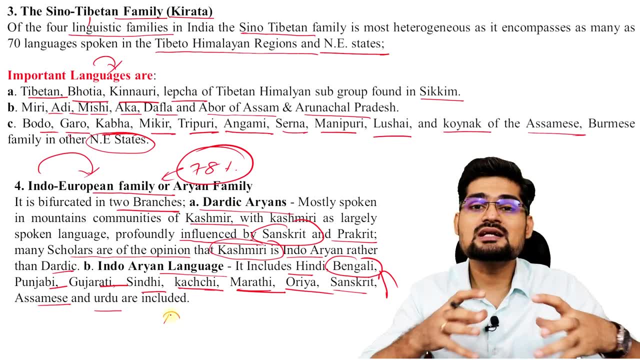 of language, or we can say linguistic plurality in India and the emergence of Indian states after independence. these linguistic plurality played a major role because, majorly, we have have a division of states on the basis of these major languages, right? so we observe another example that how languages are geographical, travel across india from north to south, east to west. 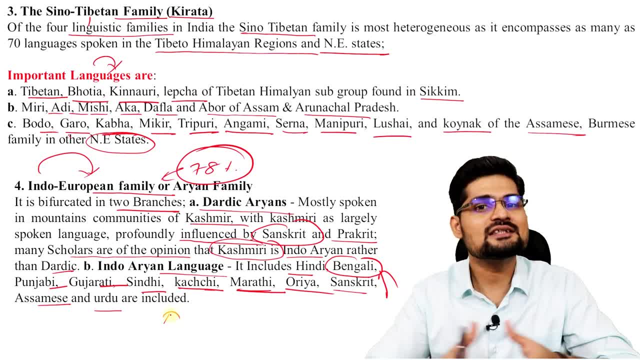 you'll find how languages changes with space. that itself is a huge example we can give for this particular thing, that how language or linguistic plurality is part of human geography or perspectives in human geography. so if you observe this map of india, this is a language map of india. 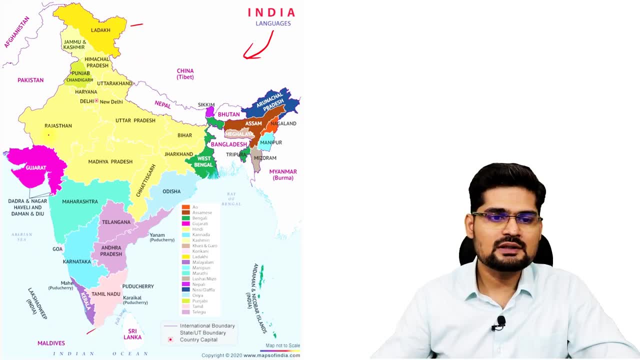 and what you observe, from top to bottom, from east to west, what we observe. there is a huge diversity, right? so this is the list. you can pause the video here and look into this map, and you can practice this map for your exam as well: that where which language is spoken, which comes from which major 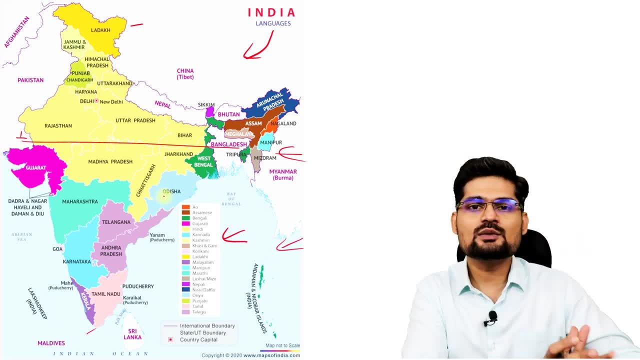 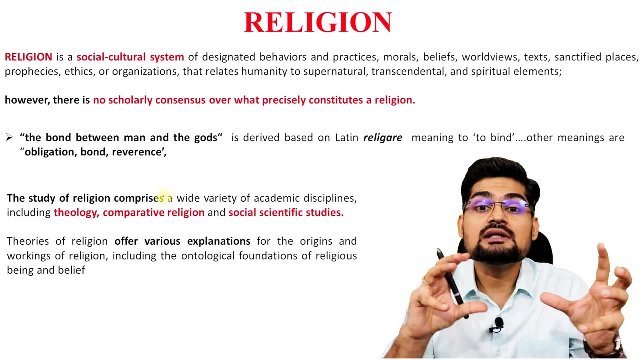 family in india. right, so that's about majorly world languages group, world family groups and the indian family groups of languages. now the next thing that we need to learn here is about religion: how religion emerged and how it is having also a spatial pattern, a geographical pattern across the 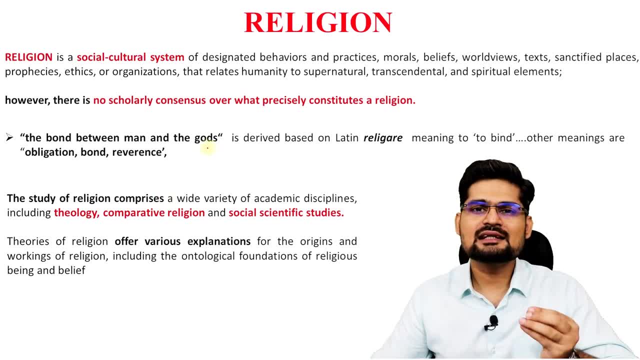 globe and india. so first of all, before going into the spatial pattern, let's understand the basic points where religion is concerned. so religion is basically what it's: a socio-cultural system of designated behaviors, practices, morale, belief, world views, texts, sanctified places, prophecies, ethics or organizations, all these things. 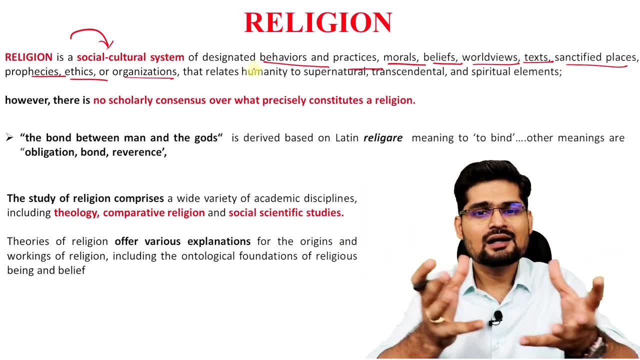 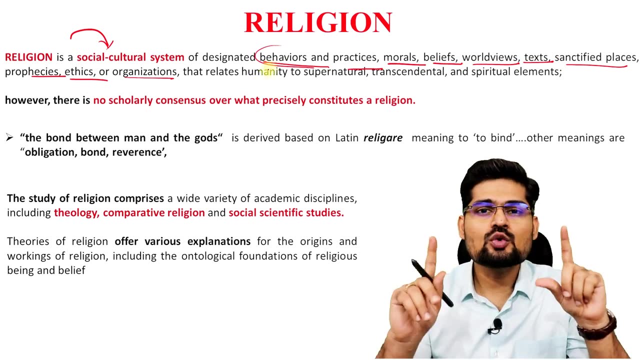 are related to religion, right? so religion is a huge umbrella under which you have several connotations which you observe here. right, so it relates to basically several transcendental spiritual elements, sometimes supernatural elements as well, right. but however, remember one point: there is no single definition of religion, right? it's a multi-cultural aspect, so it has a multitude of 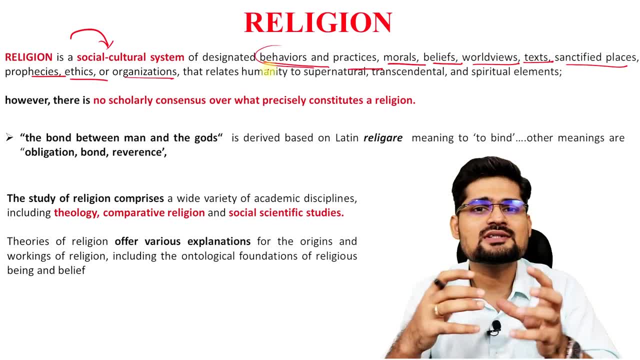 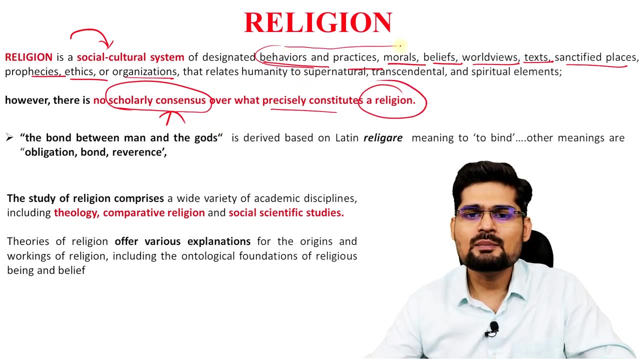 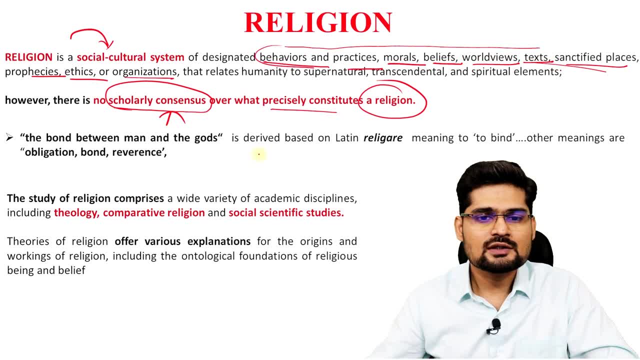 brother, one particular religious group has been lesser thế nod행. you may not know that there is no such thing now. when we practice religion, religion ultimately is what we define as the Iraq of religion. there are things that we father journalists those are: make people bind into one right to make them a group right. that's what the basic meaning of 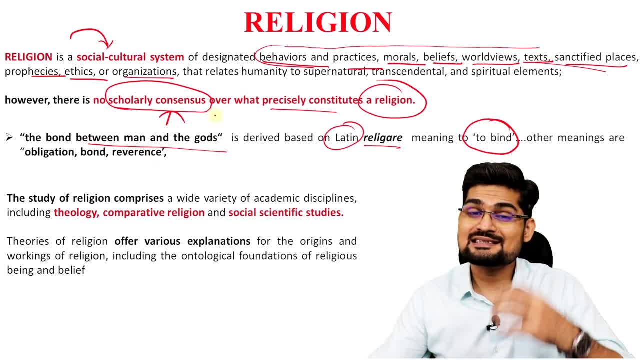 religare is. so there is a bond between man and gods that is discussed in religious lines, which binds people into one. other meanings are also there, for example obligation, bond or reverence. these are basic english meaning derived from latin right. so what we observe, the study of religion, 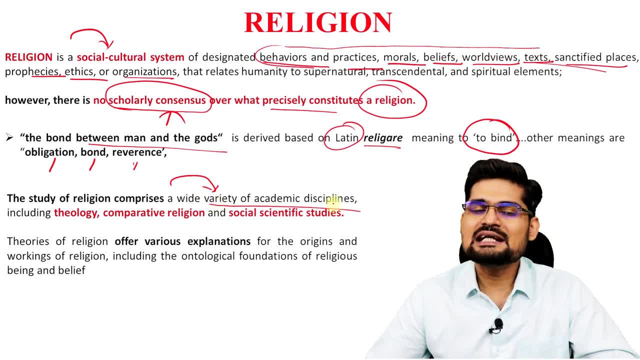 basically comprises of what it comprises of wide variety of academic disciplines, and if you have heard of these disciplines- theology, comparative religion, social, scientific studies- right. so these are major aspects of academics under which various religions, their origin, their evolution, their various factors, their connotations, their belief systems, their cultures are being studied under 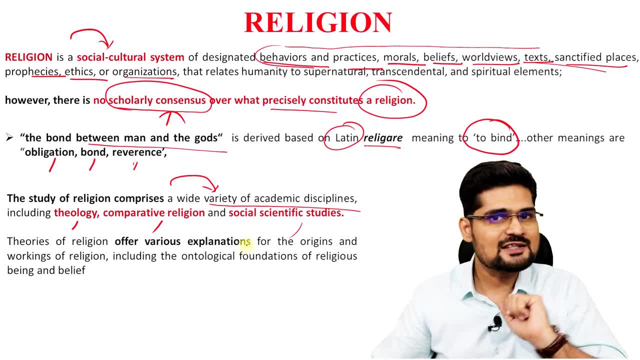 what practices it occupy the spaces. right, so that is being studied in these branches, and theories of religion offer various explanations for the origins and working of the religion as well. right, so, when we go into the academics of religion, we understand how these explanations have shaped up, and that's a purely human attribute, if you observe. right, a human creation. so it. 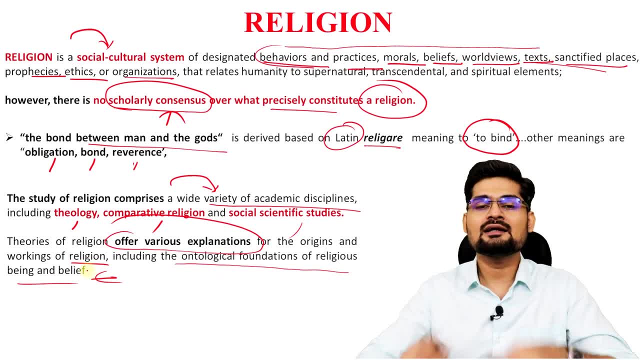 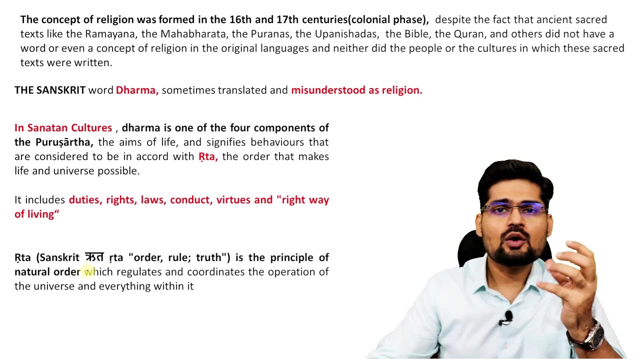 includes the ontological foundations of religious beliefs and being existence, right. so when we say ontological belief, it means what is that exists? this particular question right? this is answered under this particular segment of religious studies like theology, comparative religion. right now, let's understand one more thing here: that the concept of religion is not very old. why? 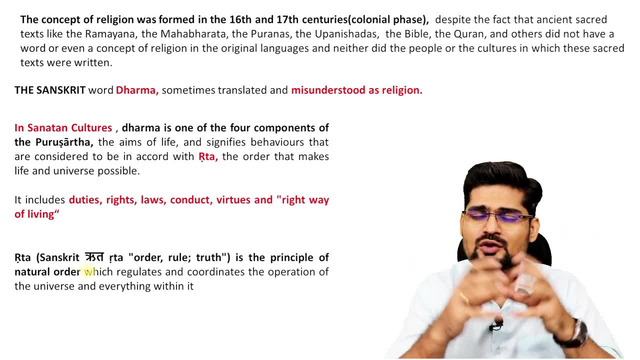 many people think that religion concept is very old. no, remember, this religion concept was formed just in 16th, 17th century when colonialism was dominating the world. so what was before that? there is important thing here to understand that, despite the fact that ancient sacred texts like 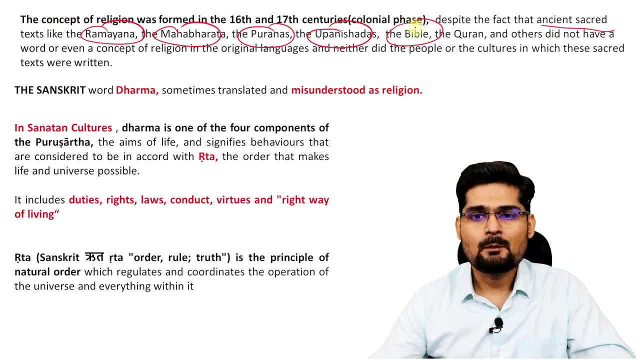 ramayana, mahabharata, purana and many other things like that were formed in the 16th and 17th century. there is a concept of religion that is not there in the originality. this is a construction of colonialism, which dominated the world, and this word, religion, was now across the cultures, right. 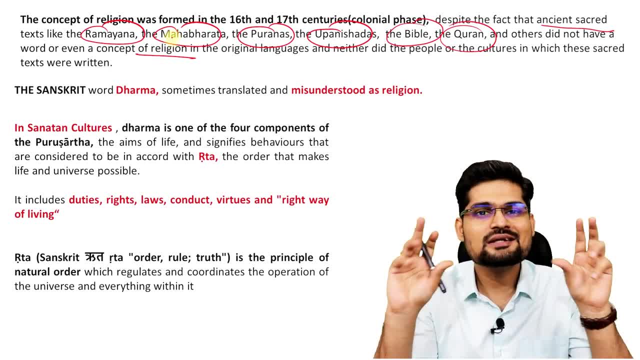 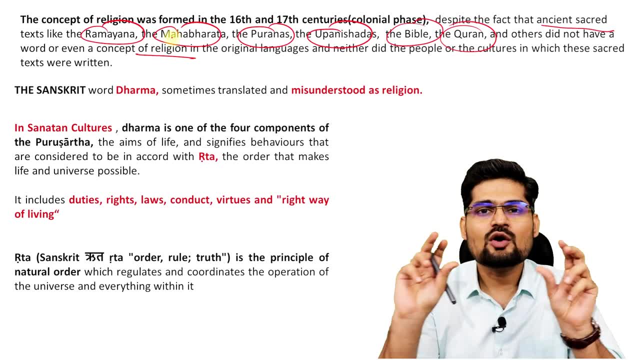 that's how people started to say this word religion. earlier the word religion itself did not exist, isn't it so? many times? in india, if you observe, religion is taken as an official word for census, right, but understand that many times people get confused between two words called religion and dharma. 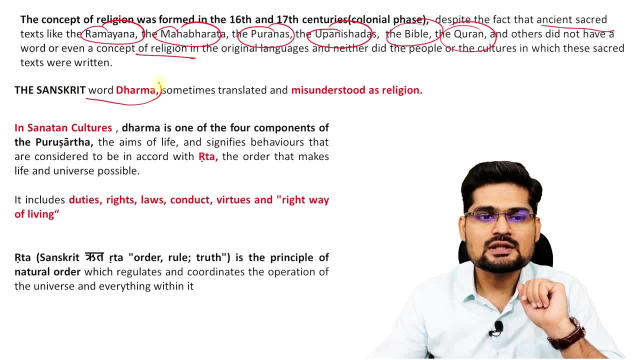 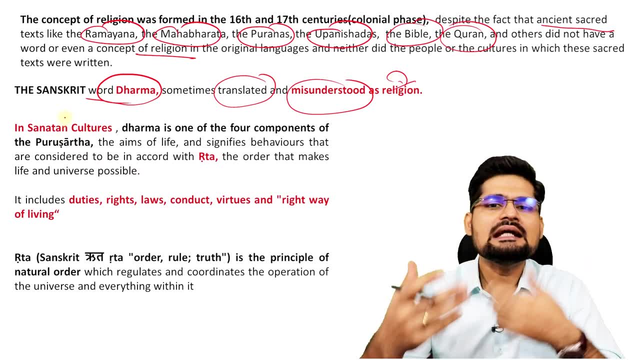 now there is one interesting take here: that sanskrit word dharma sometimes translated and misunderstood as religion. right, these are two different things, but we take it interchangeably, we use it wherever we want, but the idea is that a dharma was never talked about and never. 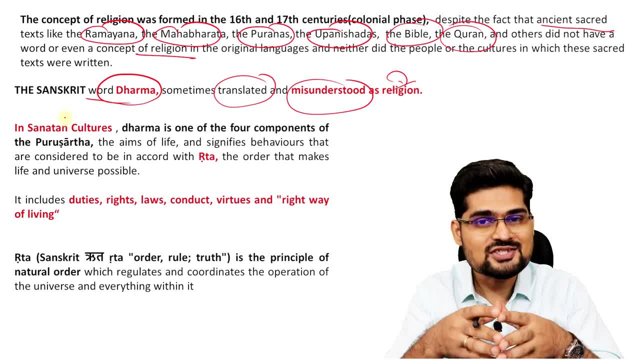 represented in the texts or in the oral traditions as a religion. right in Indian Context if we say right, because the religion concept itself is western concept that came to India through colonialism. right so in sonLC that we say that is two practices. right, so Dharma is one of the four. 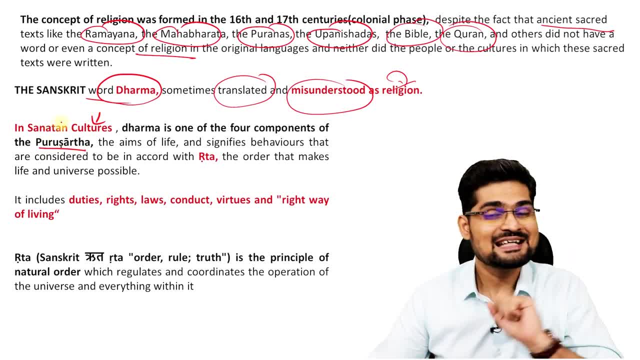 components of poor shots, which has been explained in various texts, in various puranas and Okay, right, so the aim of life signifies behaviors and are considered to be an accord with the secreta. Okay, so we've givenahaha is always presented with the foreign narrative, which means: and the other cheese is related to ludzie such as rita. so what is this? is lived wisdom, natalizing Hogam or spiritualism. therefore, Star 입니다 Bhagavad Gita. 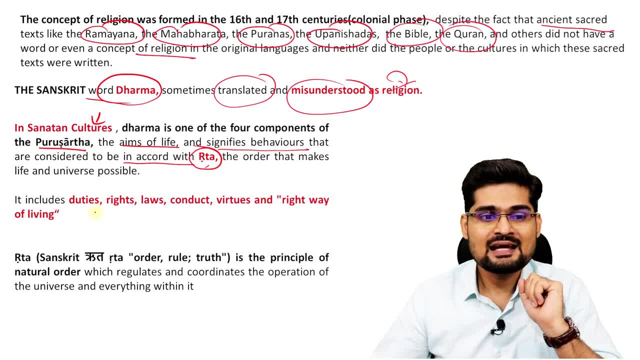 rita. this rita is the order thing that we say, and it includes duties, rights, laws, conduct, virtues and right way of living. so in india, dharma was understood in these words. if you want to explain dharma in certain words, in certain vocabularies, how can you explain? you cannot explain dharma in. 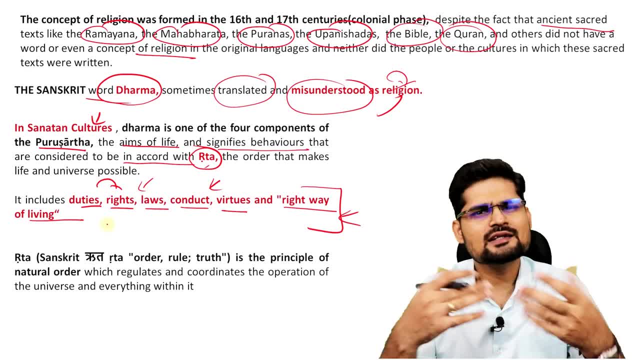 terms of religion, right, you can use it interchangeably. it is being done interchangeably even by census of india. it gives you a category across population in terms of religion, right, but in india, if you observe the old text, the word religion does not exist. dharma exists and dharma. 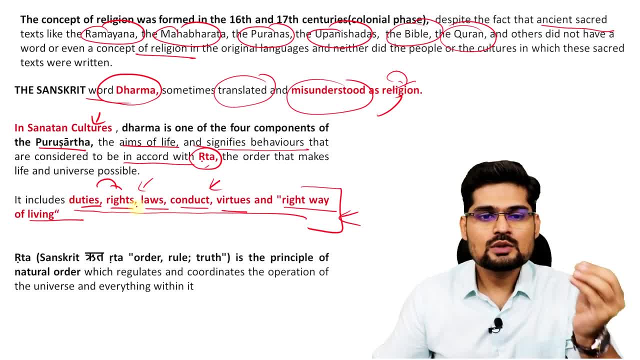 has been described in these meanings. so this word rita, right of which dharma is one part, remember this. rita is basically order, rule or truth, which is basically a principle of natural order. so basically, dharma is talking about orderness, it's talking about a rule. 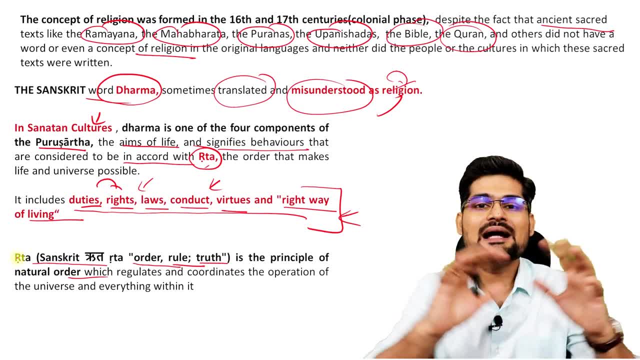 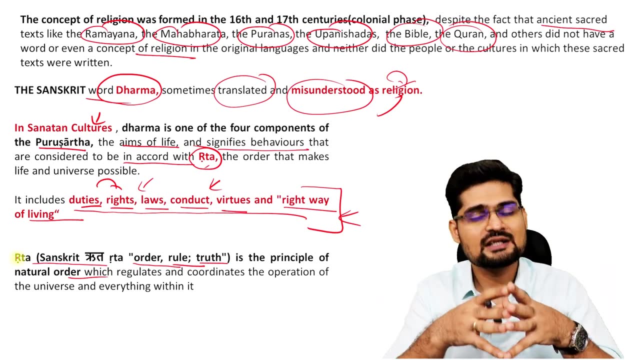 about a conduct, about a virtue, rather than just binding people together. right, it's talking about multiplicity in indian context. right, that is the clear-cut difference between a dharma and religion, which is important to understand, at least for textual connotation, because there are various interpretations of religion and also there are various interpretations of dharma across cultures. 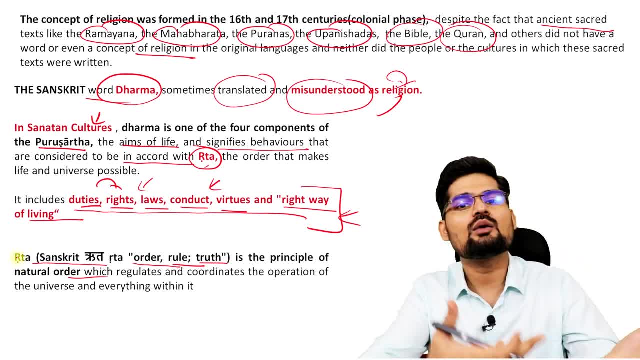 right, but to understand basic word meanings and how it came to us and how we study this in geography as a spatial pattern across world and india. it's important to understand now if you observe the word religion across india in terms of census of india, as i was saying. so what does? 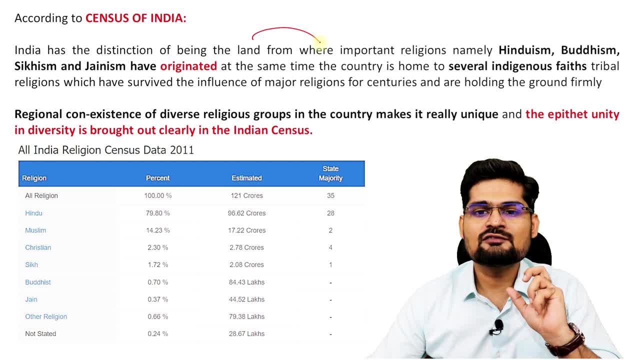 census of india say, india has a distinction of being a land from where various important religions, namely hinduism, buddhism, sikhism, jainism, have originated. so what we observe- regional coexistence of this diverse religious groups in the country- makes our country really unique. we say unity and diversity. right, and it's the epithet that we use always. that is. 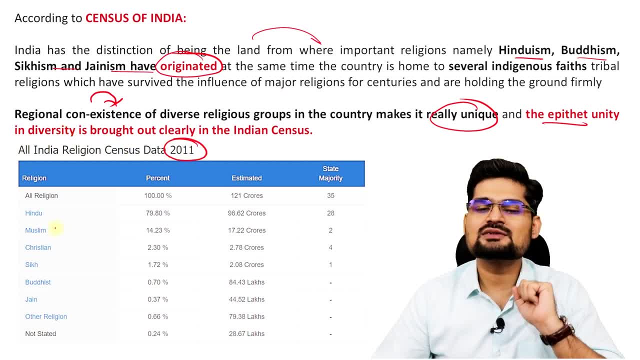 unity in diversity, right. and if you observe the last 2011 census, it gives us what religion in one column, percentage here and estimated population. so you observe hindu, muslim, christian, sikh, buddhist, jain and others, right, this is the several category of religions. if you observe indian context and 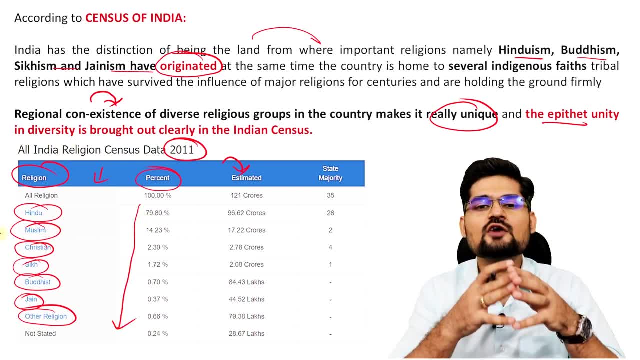 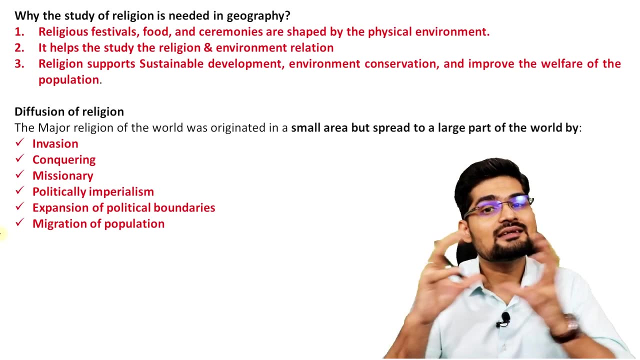 their percentages are given you right. so what we observe, the census of india officially defines these particular religions that exist in india and that's important to learn here. but it's important not to confuse between the word dharma and religion, right? that's what you should understand as a textual analysis. now why? 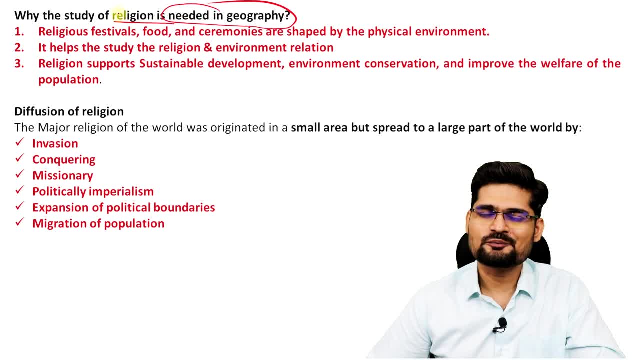 we study religion and what is its need in geography here? why are we talking about religion here? why did we talk about language? because, remember, this is not just about one point of the textual analysis: culture. it's also about space and its attribute, created by human beings, part of human space, that's. 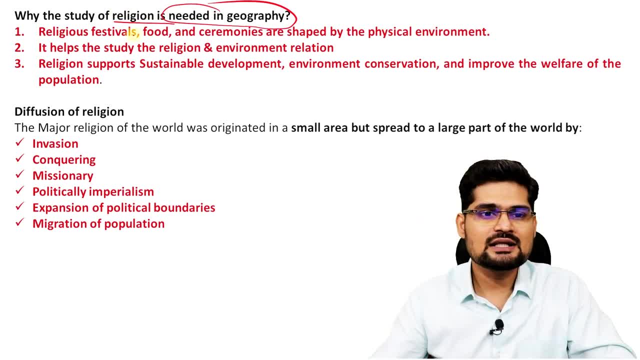 what we understand here as human geography attribute right. so religious festivals, food ceremony, are shaped by physical environment. it helps study the religion and environmental relationships, and religion supports sustainable development, environment conservation and improve the welfare of population as a basic premise, isn't it? that's why we understand that religion is not? 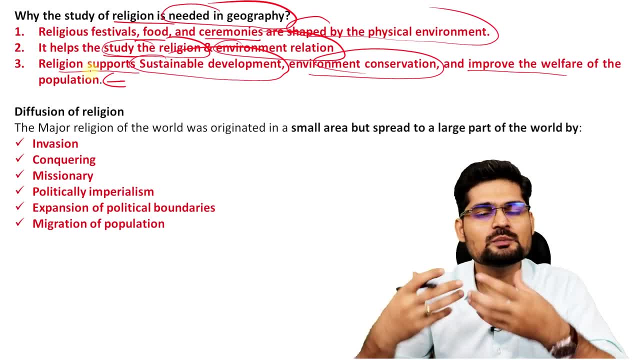 just part of a particular faith or a particular people to believe or practice, but it's also in relation to human beings milieu that they construct, isn't it? so that's why we need to understand. so, when we understand this, there is another thing here: diffusion of religion across the world. and 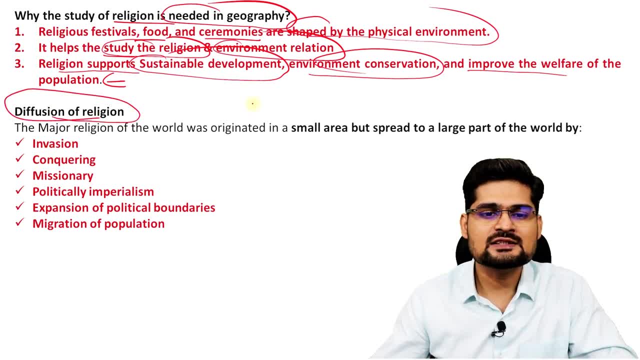 across India. so if you see diffusion of religion, it means from a center where the religious thing emerged or originated, how it actually diffused across the space. so what are the processes behind it? now, if you learn geographical history here of religion, there are several factors that we need. 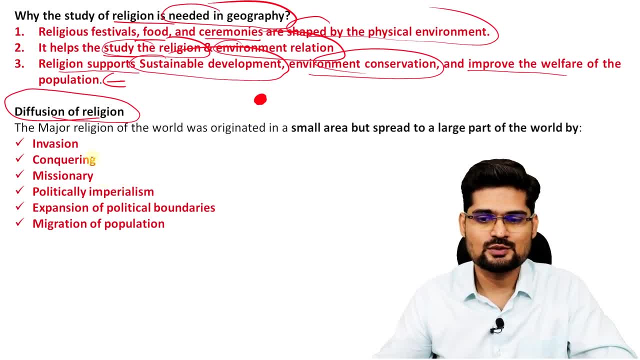 to understand which is behind this diffusion of religion across the world. so, invasion, conquering, missionary politically, imperialism, expansion of political boundaries and migration of population. these are several factors across the religions of the world. if you find that's why these religions expanded from the source of origin, on the basis of these factors, isn't it so what you observe? 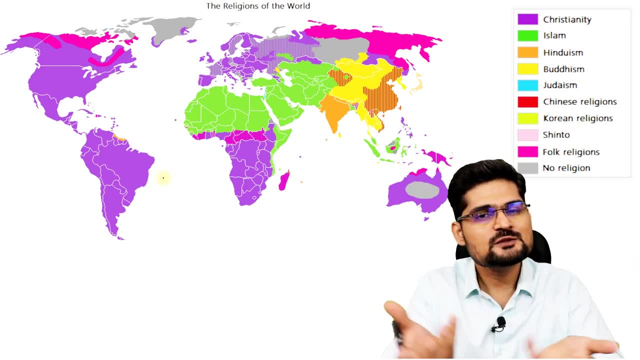 again you. in religion, like language, we have a colorful spatial pattern of the globe, right? so what you observe, look here, this one is Christianity, Islam, Hinduism, Buddhism, Judaism, Chinese religions, Korean religions, Shinto, folk religions, and there are certain places where still we don't have any. 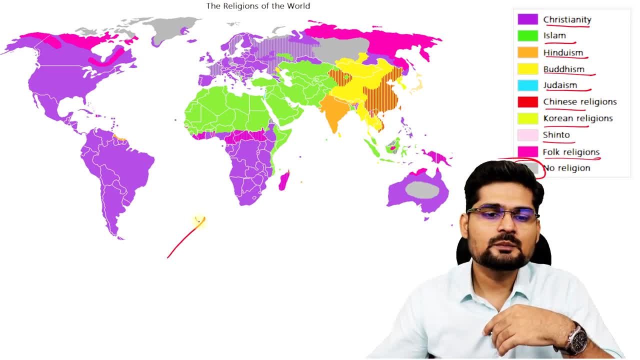 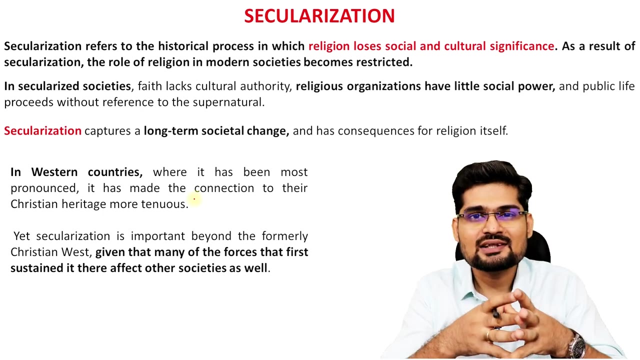 religion as such, right? so this is this colorful picture that tells us that religion also is spatial in nature. it is regional in nature, isn't it? that's why it's geographical in nature, right? so now, the last point in this lecture is secularization. and what does it mean? 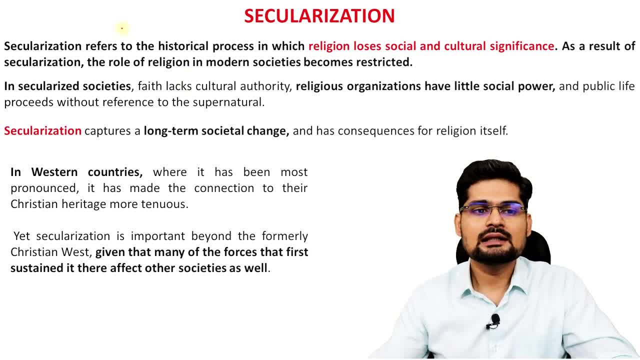 so when we say religion spread across the world, now it's important to understand what is this process of secularization? so this is a process in which religion loses its social and cultural significance. so what happens here? here the societies, or we say modern societies- makes restrictive policies about practicing religion right, and we also have a process of secularization. 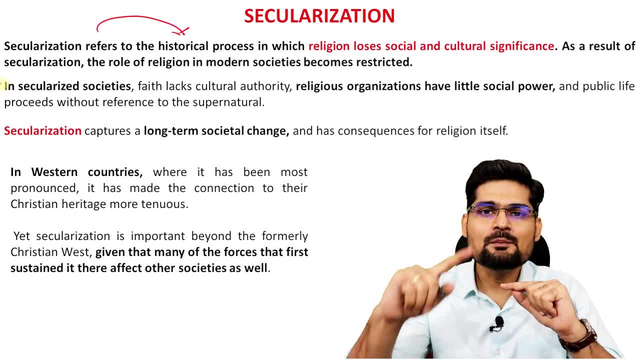 it means basically what? it means that one cannot impose their faith of religion on the other. so when we say there is everyone that is important, not just one religion is more important, that is a secular behavior, isn't it so? what we observe here in secularized societies, what happens? faith? 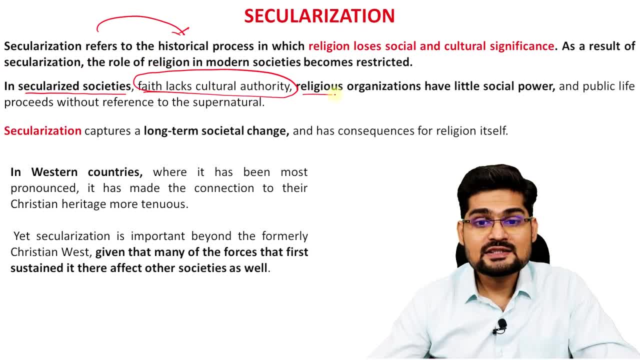 lacks cultural authority. one thing then: religious organizations have very little social power and also public life proceeds without reference to supernatural or religious connotations of various kinds. so secularization is basically about modernity, the long-term societal change, and has a consequences for religion itself. by the end of 19th century it became 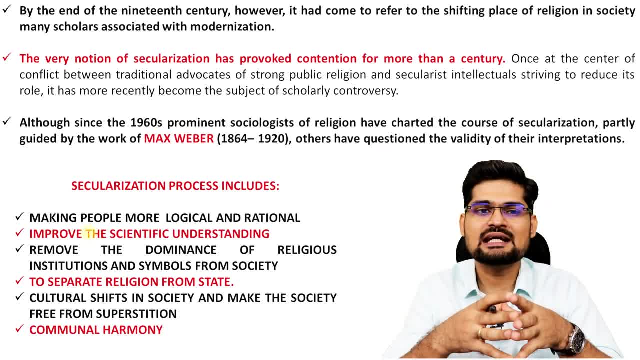 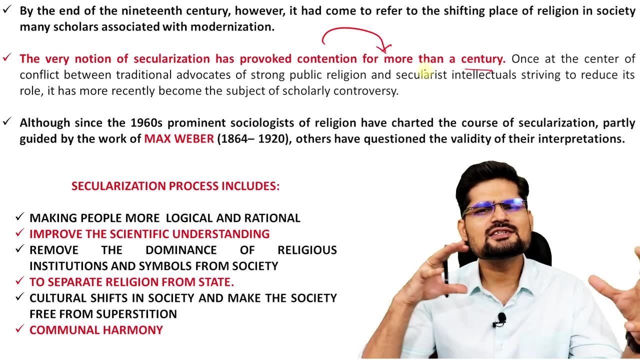 one of the reference of shifting places of religion in society by scholars, and they said: to be modern, we have to be secular. this was the definition right. so the very notion of secularization has provoked contention for more than a century and there is a huge debate across India, across world, on what should be the path of modernity. shall it be religious? 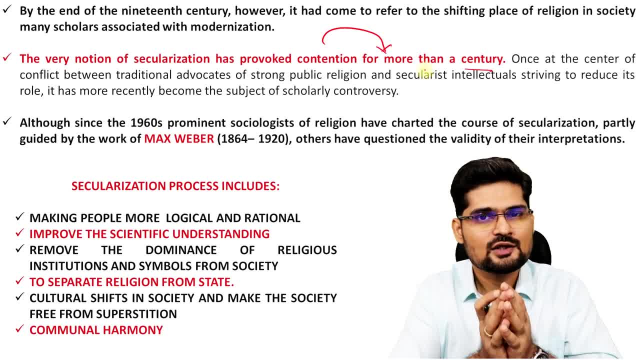 path, faith part, or shall it be secular path which is more important, right which is more sustainable? so remember there is a scholar called Max Weber. he also talked about this process of secularization and his work is very interesting in terms of the course of secularization through history, which 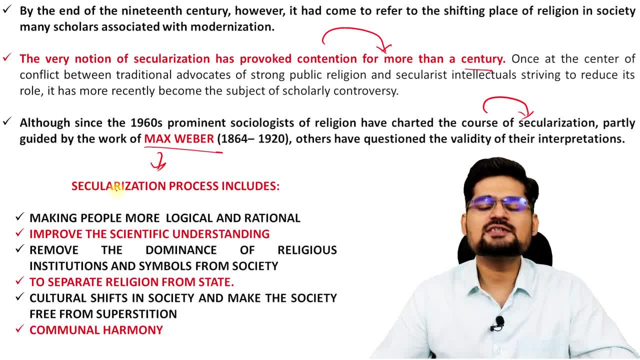 has also been criticized by many other scholars. so secularization process includes these points that you can remember. in short, right. so making people more logical and rational. that is about being scientific, being evident, not talking about supernatural or metaphysical right. improve the scientific understanding, then remove the dominance of religious institutions and symbols. 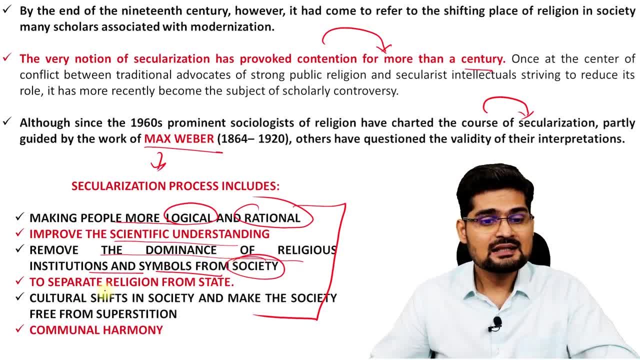 from society. that is one aspect of being secular. then, separate religion from state. very important aspect is that state is for everyone. religion is for the believers and practitioners of that religion- Right. and then cultural shifts in society and make the society free from superstition- right. and communal harmony: right, because many times because of religious tensions, communal.